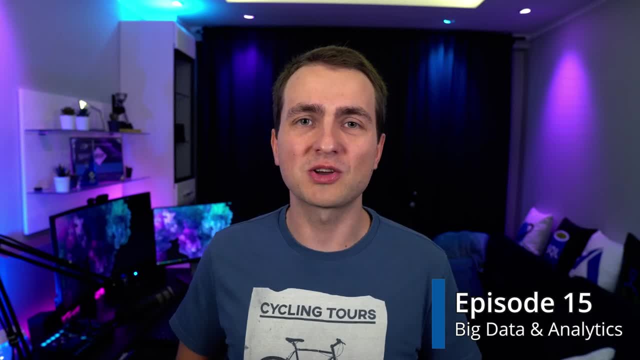 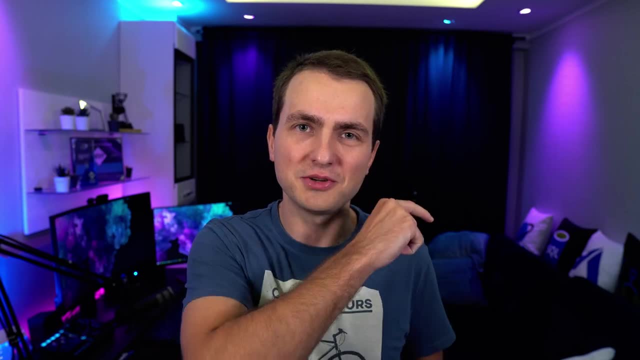 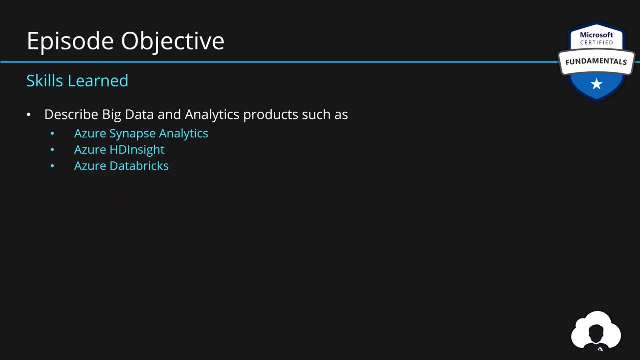 Hello guys, welcome back. it's Adam, and in this episode we'll be focusing on what is considered big data and which services in Azure help us process and analyze those kind of data sets. Stay tuned. As part of episode 15, we will learn about three Azure services. This time it's going. 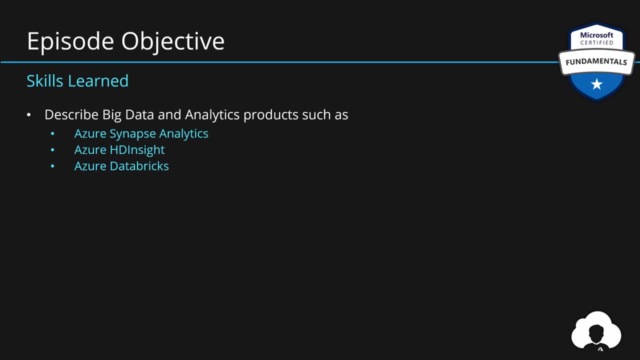 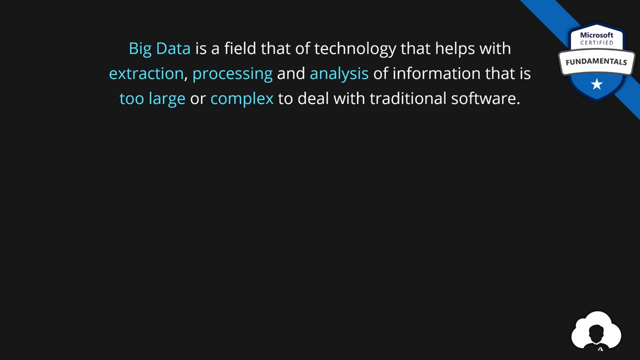 to be Azure, Synapse, Analytics, HDInsight and Databricks. But before we move to those services, let's backtrack a little bit and let's talk about what is considered big data. Big data is a field of technology that helps us with solving typical challenges around extraction, processing and 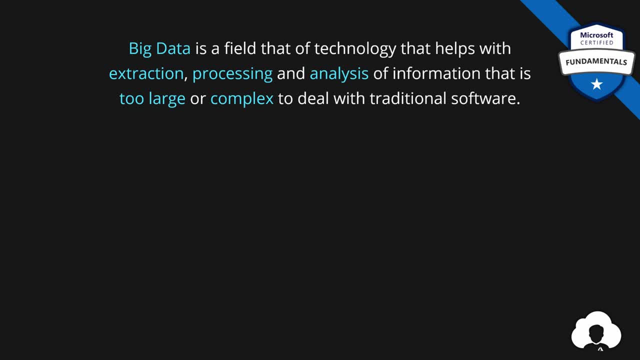 analysis of our data sets. But typically, in order to call something big data, certain characteristics has to be met. The first one is velocity. Velocity means how fast is our data arriving? how fast, how often do we need to process that data? Are we processing that data in batches, or maybe in? 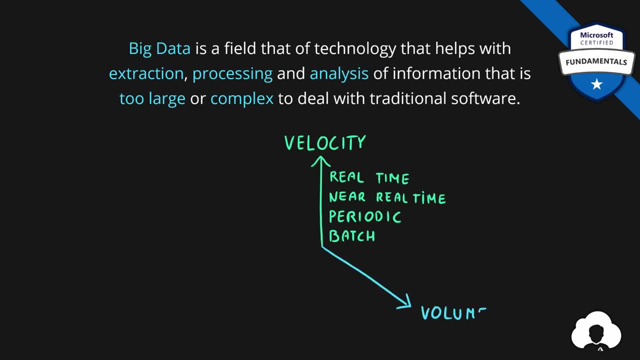 in real time. A second characteristic is volume. So are we talking about megabytes, gigabytes, terabytes or even petabytes of data? And the third one is variety. Variety means that how structured is our data? Are we talking about tables or databases, or maybe something very 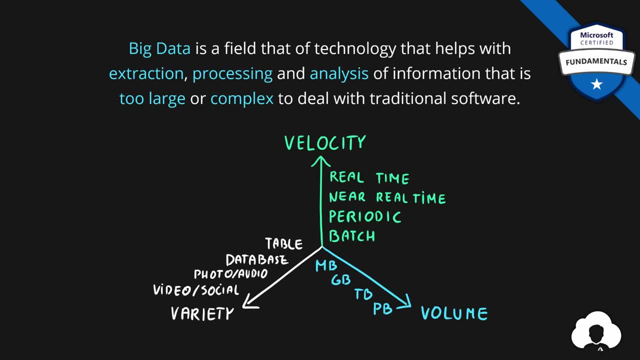 complex, like video or social media information. Based on these three characteristics, we can define whether this data is considered to be big data or not. But as soon as we go high on one of those vectors, one of those characteristics, traditional softwares will not be able to. 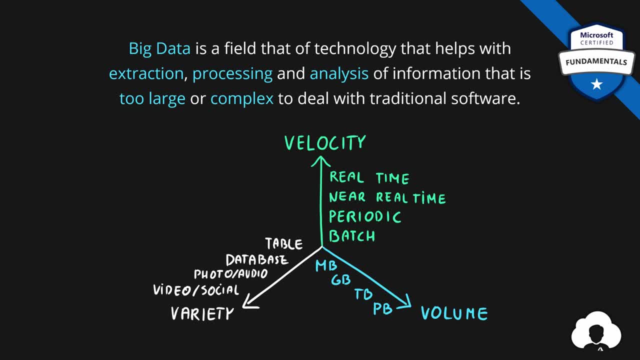 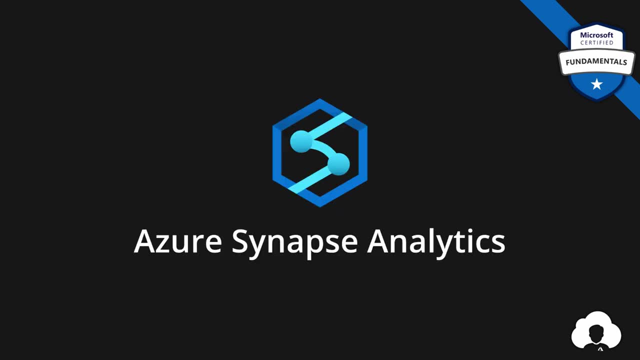 process this kind of datasets, And this is how big data technologies came to be. They were specifically designed softwares to help us with those kind of challenges, Which brings us to our first service: Azure Synapse Analytics. But in order to talk about Synapse Analytics and its 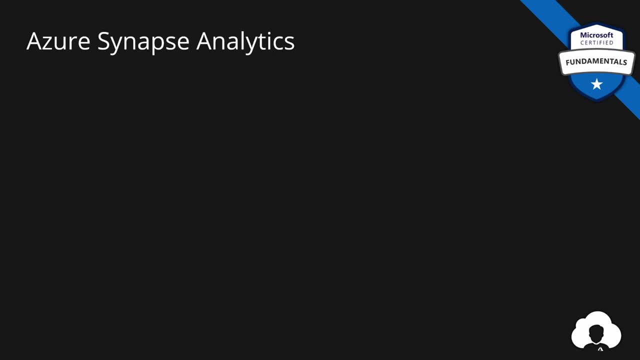 benefits. we need to talk about how typical process looks like. So let's get started. When it comes to transforming and analysis of our data, most data engineers will start their process by identifying where is their data, whether those are flat files, some web services. 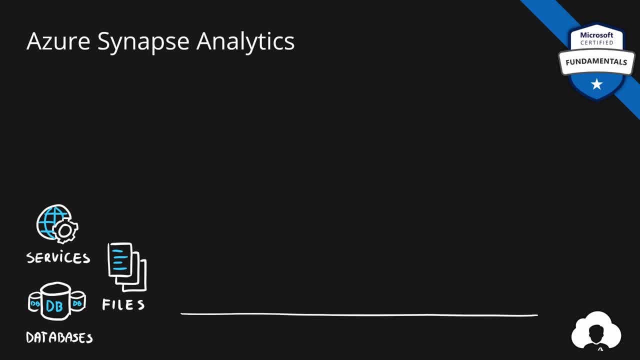 or databases, And from there a typical development process starts. So developers will first need to ingest the data from their sources to the cloud, Then they will need to transform those datasets and store them somewhere And, after storing the data, expose this to other tools like reporting. tools so that business can use them, And then they will need to transform those datasets and store them somewhere. And then they will need to transform those datasets and store them somewhere. And then they will need to transform those datasets and store them somewhere, And then they will need to. 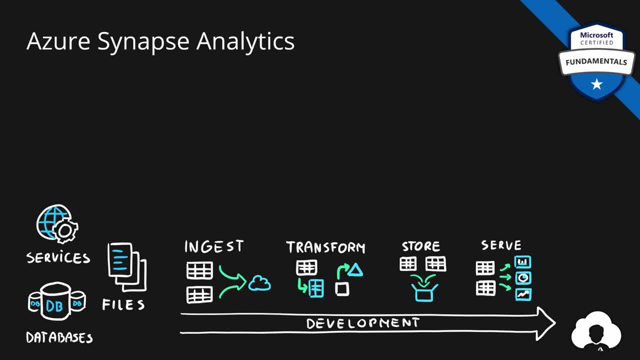 take insights out of their data and make good business decisions, And Azure Synapse Analytics helps with all of those steps. First of all, by providing a feature called Synapse Pipelines. This tool helps developers to ingest and transform their data using visual workflows. 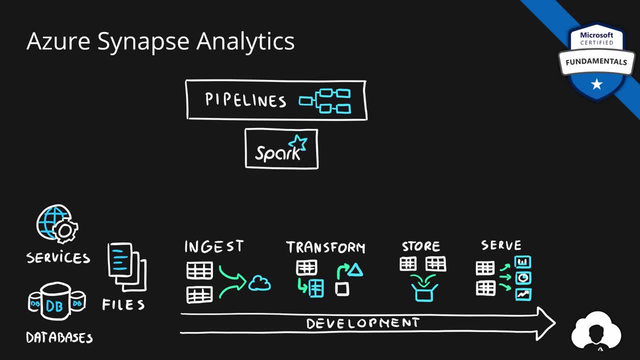 Additionally, Synapse Analytics comes with embedded Apache Spark, a leading technology for big data analytics and transformation. In addition, there's Synapse SQL, a massively powerful and powerful tool for data transformation, And it's also a great way to effectively parallel processing database clusters based on a popular SQL server. This feature helps. 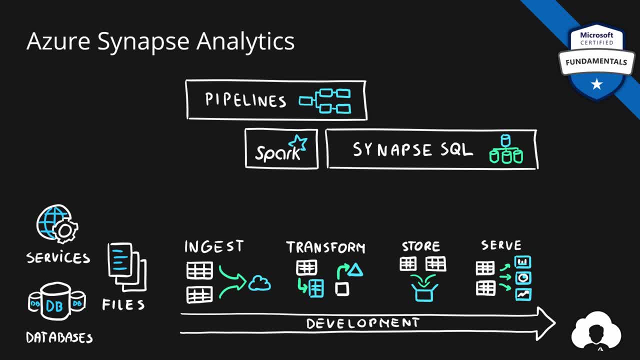 with transformation using typical SQL queries, storing of your data but also serving it to your reporting clients. And all of that is baked into something called Studio- Synapse Studio- which is a unified experience to manage all of those tools and features and perform all of your. 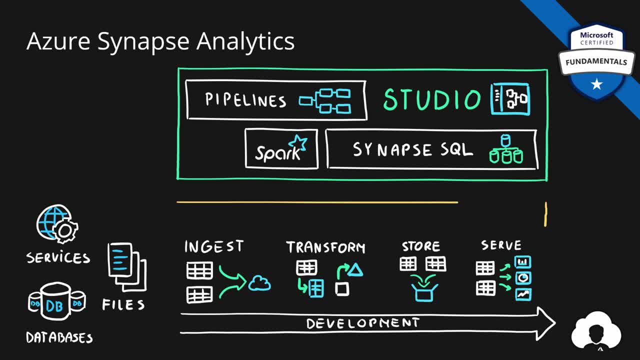 data transformation in a single place, And all of that is nicely integrated with another Azure service called Data Lake, so that ingestion, transformation and storage of our data can be also done directly on the Data Lake. To summarize, Azure Synapse Analytics first of all and foremost. 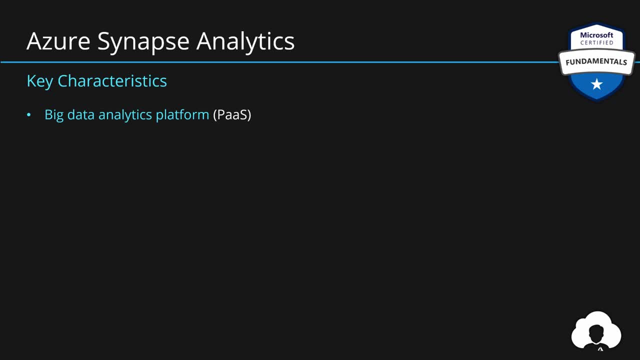 is big data analytics platform. It's a platform as a service offering in Azure allowing users, data engineers, data scientists- to perform data analysis and data transformation over very large data sets, And it has multiple tools baked in tools like Apache, Spark for efficient. 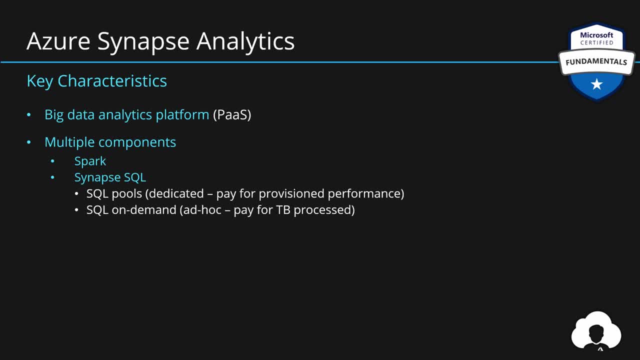 big data transformations. Synapse SQL, which allows us to use SQL server familiar tools with massively power processing design with dedicated or ad hoc capacity. You also have Synapse pipelines, which allow you to visually build your ingestion and data transformation workflows. And all of that is combined into a single studio experience, a unified experience. 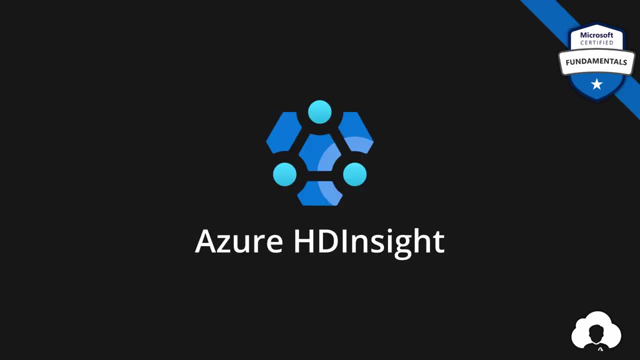 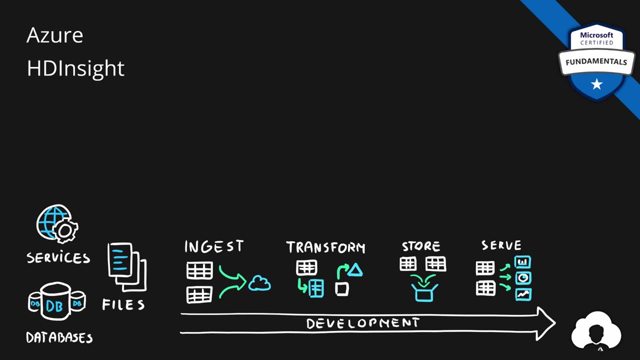 for your data transformation needs. Next on our list is Azure HD Insight. As we were talking about the typical development process, HD Insight can also support pretty much every stage of that process by providing so-called big data clusters, And when it comes to HD Insight, there are many. 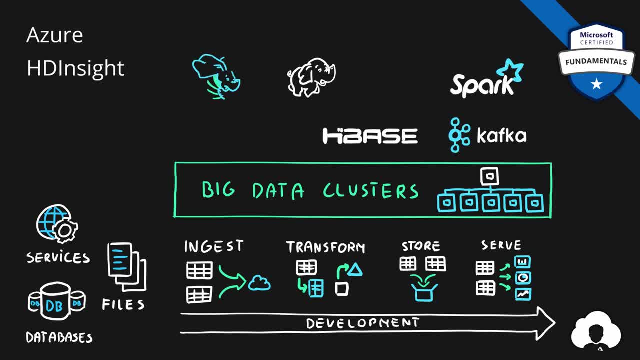 clusters available, clusters like Hadoop clusters, Spark, Kafka, HBase, Hive machine learning services or Apache Storm or many others. In general, the idea of the service is to provide you with open source big data technologies from the market. 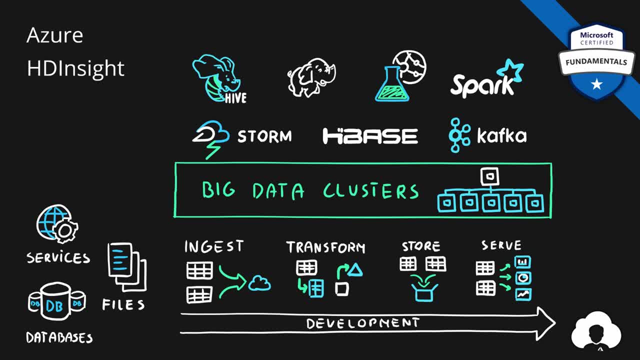 allow you to provision clusters so that Microsoft manages those clusters and you just grab the technology that you need to perform specific tasks that you need. All of these tools serve a different purpose, but you can use them in combination to support end-to-end development lifecycle for your application. So Azure HD Insight is a flexible 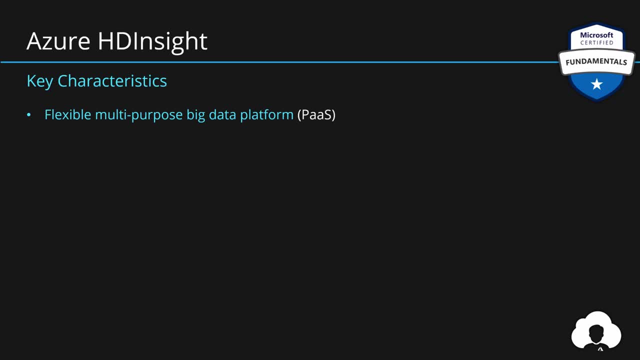 multi-purpose big data platform. in Azure, It's another platform as a service offering. allow you to choose from multiple open source technologies on the market, whether this is Hadoop, Spark, Kafka or many of the other available technologies. And, lastly, we have Azure Databricks. Azure Databricks is quite similar to 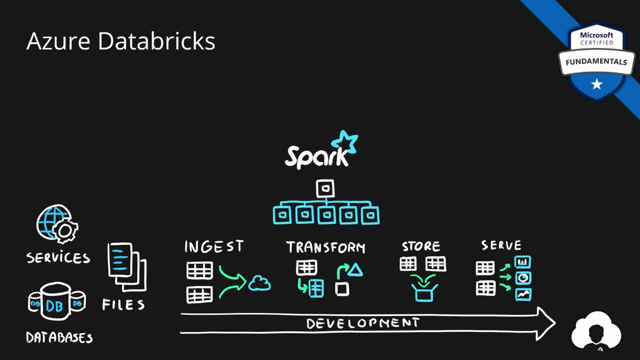 HD Insight, except the clusters that we create are based on Apache Spark and Apache Spark alone, And the main purpose of this service is to help you with data transformation at large scale, because Apache Spark is one of the leaders when it comes to performance and 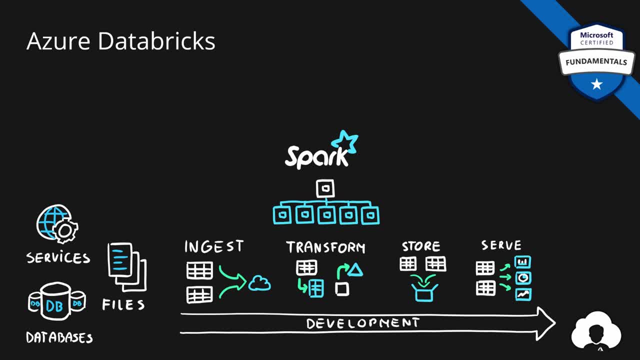 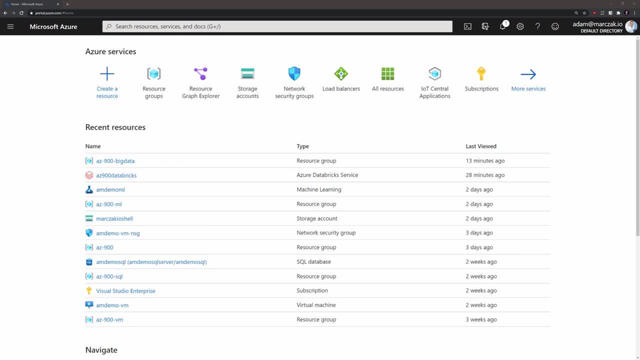 data transformations for big data. But besides the data transformation, the creators of Databricks also wanted to provide this as a collaboration platform for data engineers and data analysts, so that they have a single place where they can manage their clusters and collaborate on their data solutions In Azure Portal. I will no longer start by creating. 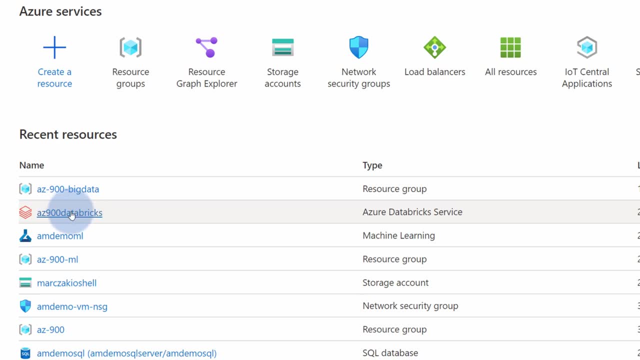 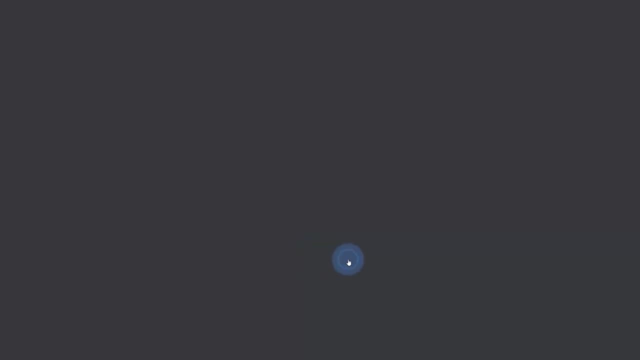 services. We've seen Azure Marketplace enough, So instead I will go to Azure Databricks service that I created previously. In here I can use a button to launch a, which will take me away from Azure portal into separate portal designed for collaboration on. 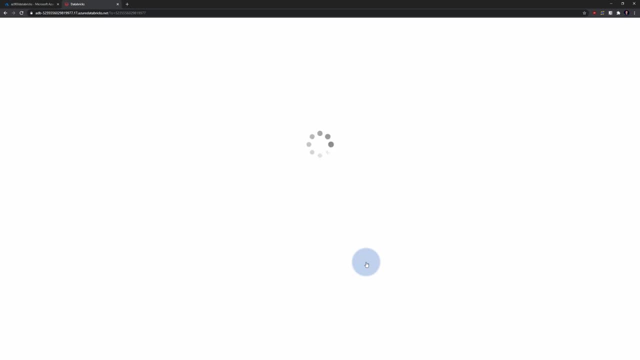 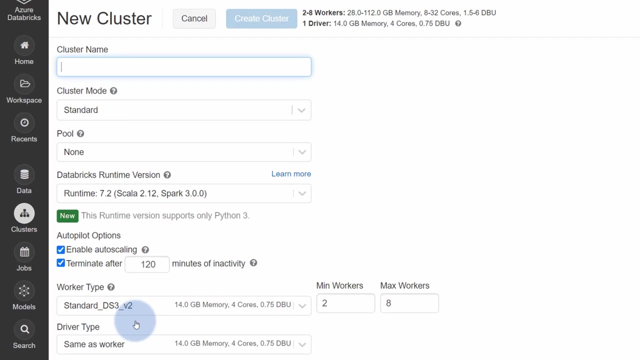 Azure Databricks solution, a so-called workspace. The first thing that we need to do inside of the new workspace is create new cluster. By opening a new cluster panel, we can specify a cluster name. In my case, this will be demo. If I want, I can tweak around some options like changing the 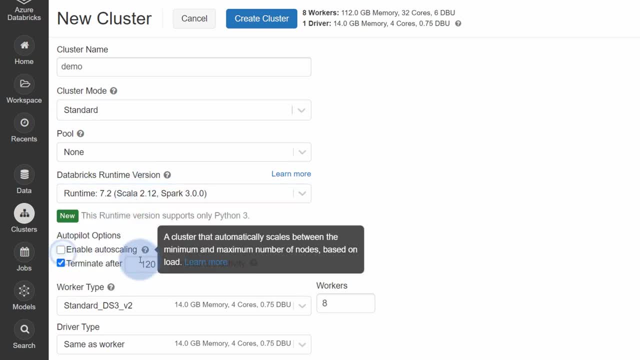 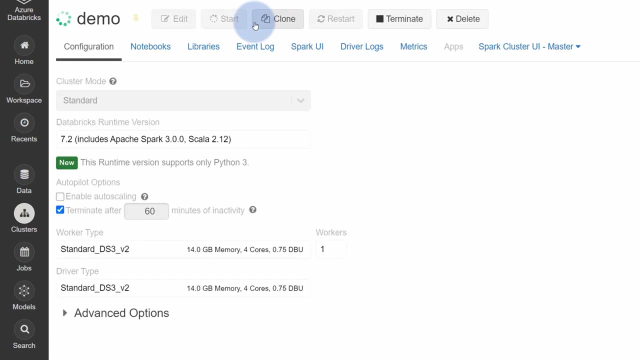 cluster type or the runtime version. I can also tweak auto scaling features and auto terminate options, which is amazing from the cost perspective. If I'm happy with all my selections, I can simply hit on create cluster and just wait. Creation of the cluster takes about four to five. 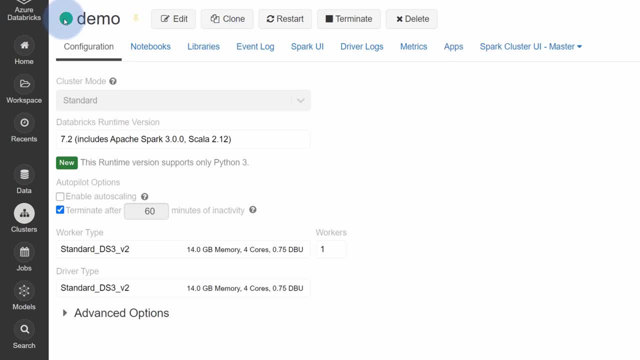 minutes. Once the cluster has been created and is in running state, we can start working. But notice how easy it was. I was just clicking few buttons and right now I have a big data technology cluster based on Apache Spark, running in the cloud and ready to be used. Now we can. 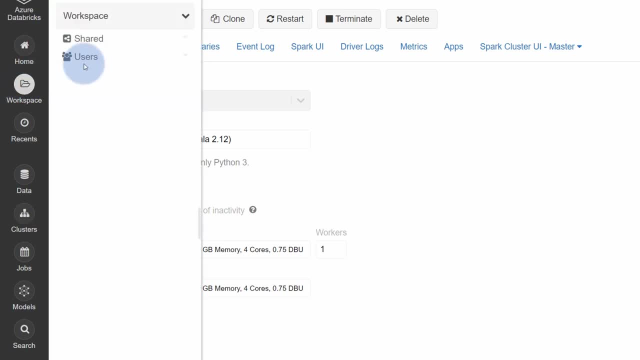 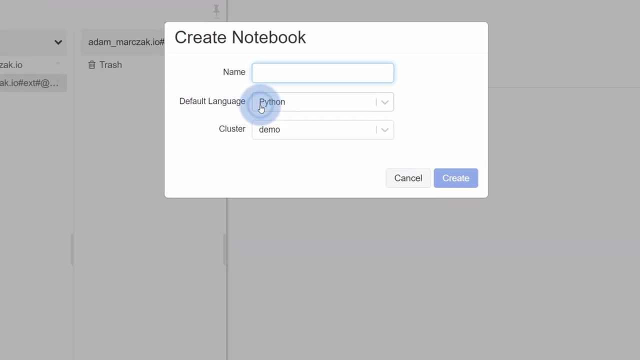 create some scripts By going to the workspace on the left hand side, where I either have my personal workspace in user section or in a shared workspace where I can share and collaborate with other users. I will go to my personal workspace, I will open my catalog and create new notebook. Notebook are simple scripts. 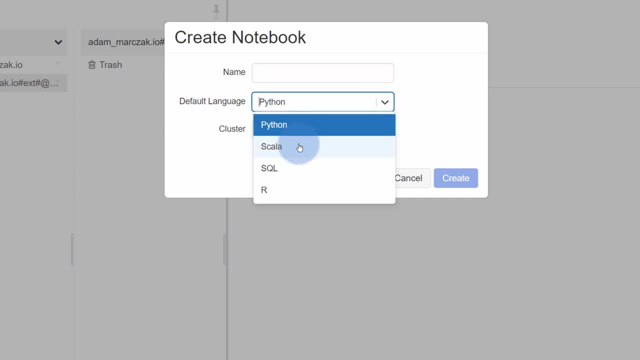 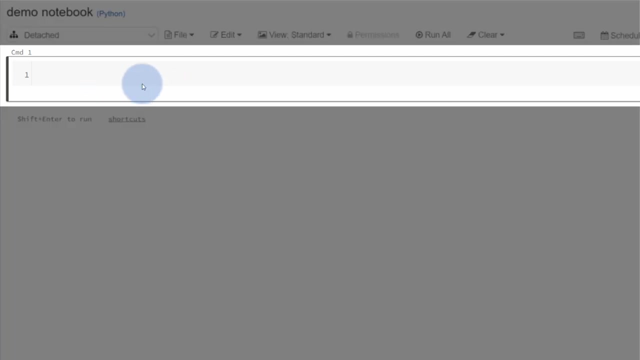 in Azure Databricks I can select a language like Python, Scala, SQL or R. In my case, I have a demo using Python and I will call this demo notebook. Inside of my notebook, you will be able to notice that there are some small text blocks here and I can. 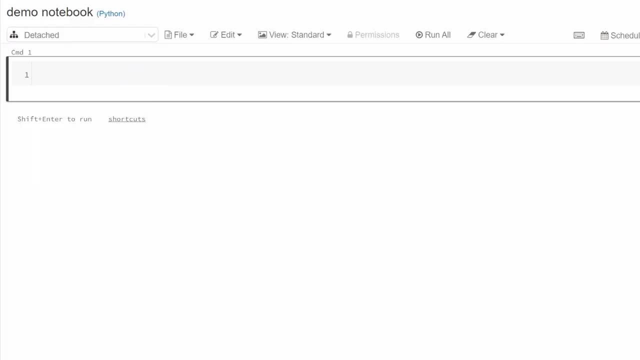 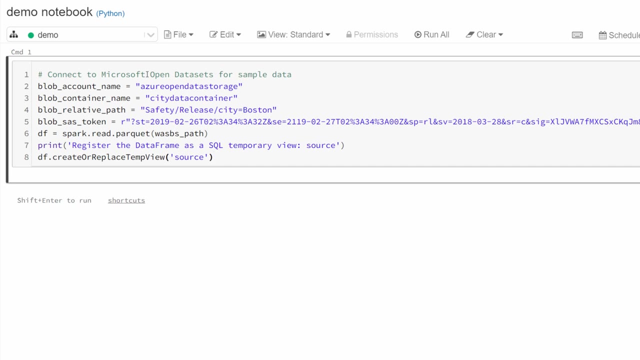 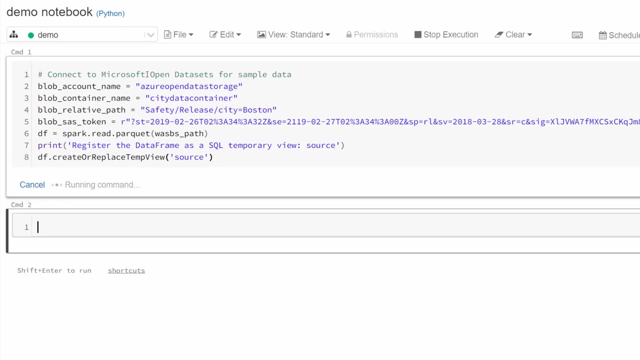 use those text blocks to write my scripts. For now I will copy paste the script that I prepared previously. For now we don't need to focus on the details of the script. What the script does is connects to open data sets from Microsoft with some sample data, and it literally takes seven. 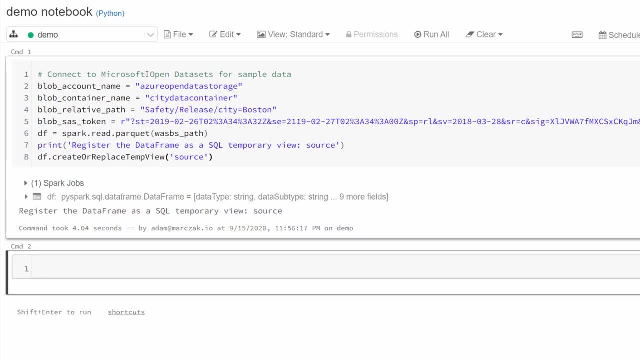 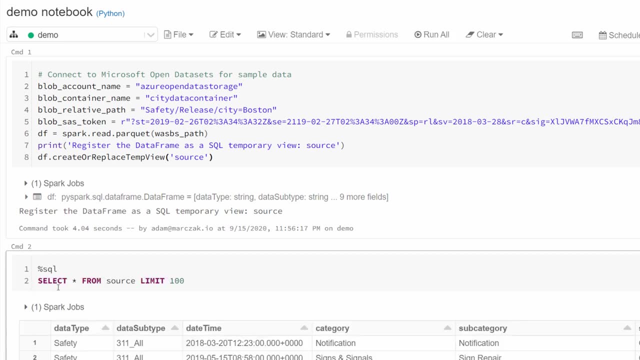 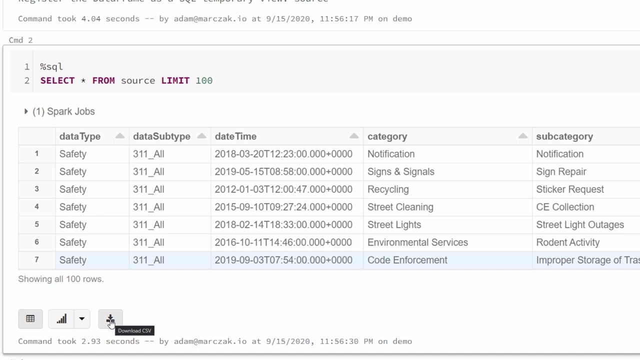 lines of code to do that. It's very simple and very straightforward. But once you put it in your database, you can use familiar SQL language. In this case it's Spark SQL, So you can use familiar SQL language to review your data and analyze it In here. you can also download this data as a CSV. 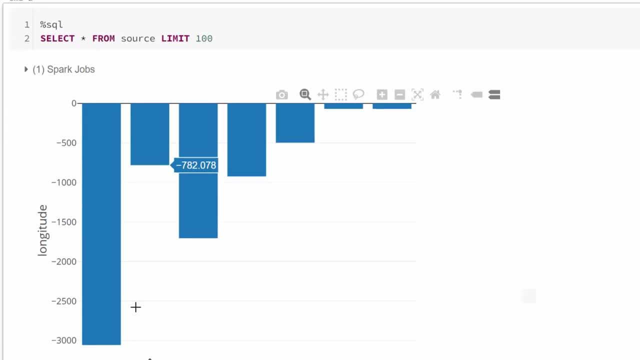 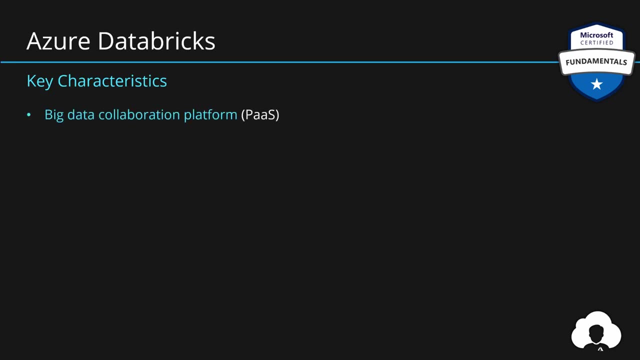 change the chart type to, to, say, bar chart, and do all sorts of data transformation and analysis based on your needs. To summarize: Databricks is a big data collaboration platform. It's another offering from Azure in platform as a service category. Data bricks is a big data collaboration platform. It's another offering from Azure in platform as a service category. 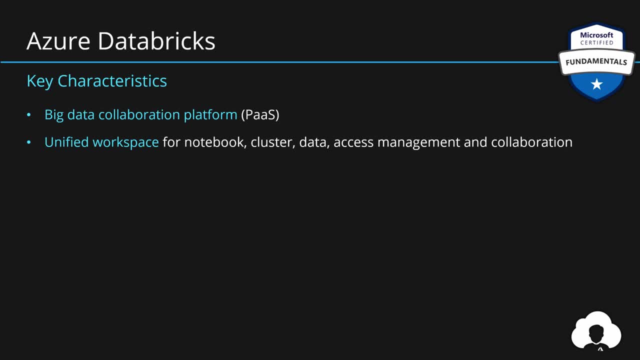 But it's really about providing this unified workspace where users can manage their notebooks, clusters, data and manage access to other users and collaborate with them, so that users can focus on their data solutions rather than on the management of their big data platforms. And it is.